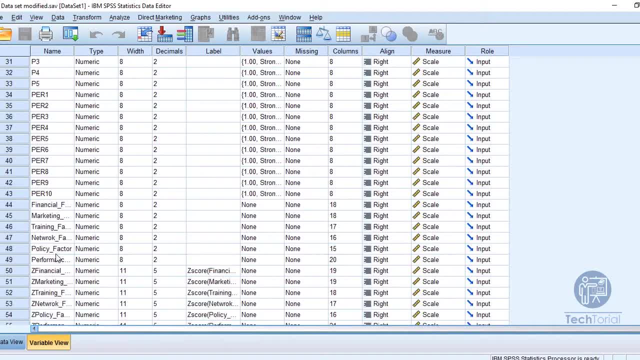 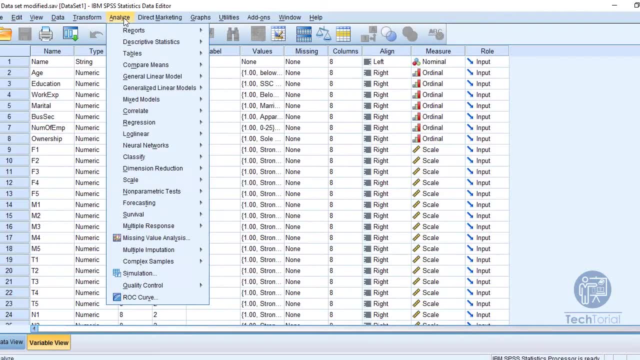 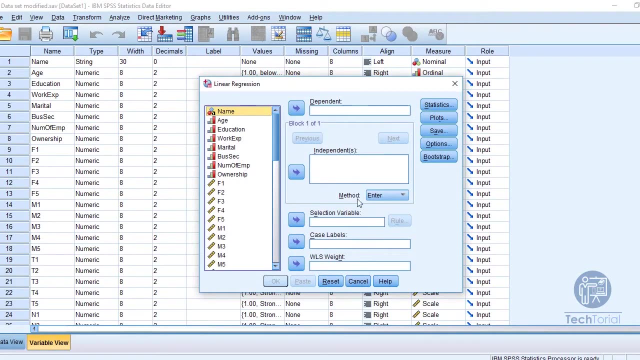 can see there are some independent variables and there are dependent variables. For the analysis of multiple regression then you have to go to the analyze, then regression and linear regression. Here you can see there are some boxes: dependent variable box, independent variable box. You have to put all of the independent variables into the independent variable box. 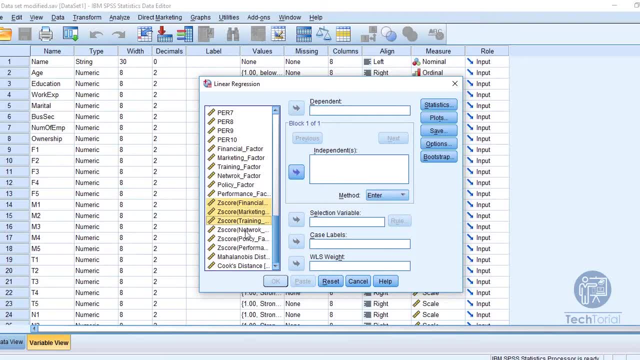 Now I am putting all of the independent variables into the independent variable box And the dependent variable and the dependent variable box. Now you have to make sure that all of the values of those independent and dependent variables must be in the standardized values, because no non-normal data can be used for multiple regression analysis. So 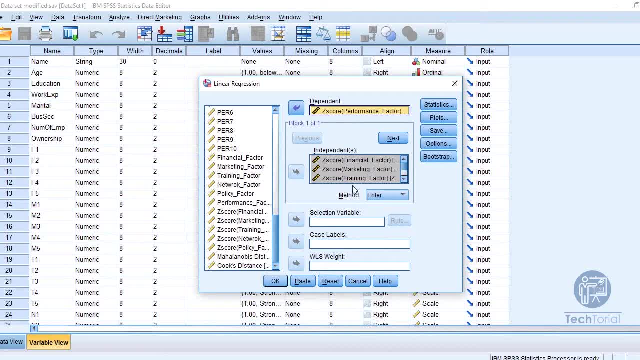 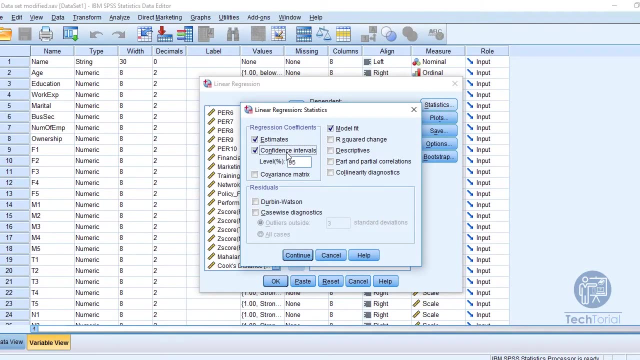 let's get to the method Now. in the method option the entered mode must be selected. Next you have to make sure in the statistics section there are estimates, the confidence intervals, model fit descriptives, part and partial correlations and collinearity diagnostics must be take in the residual. 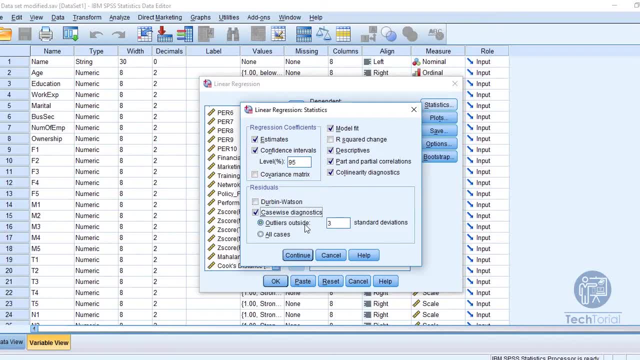 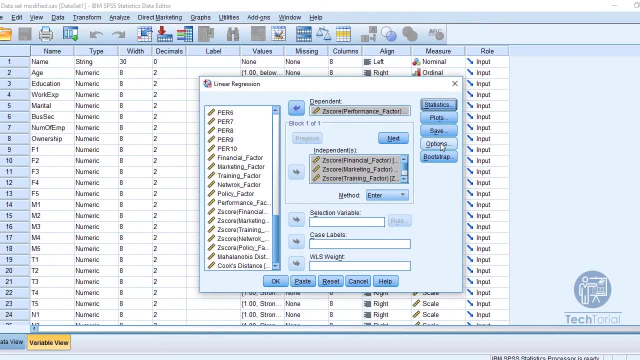 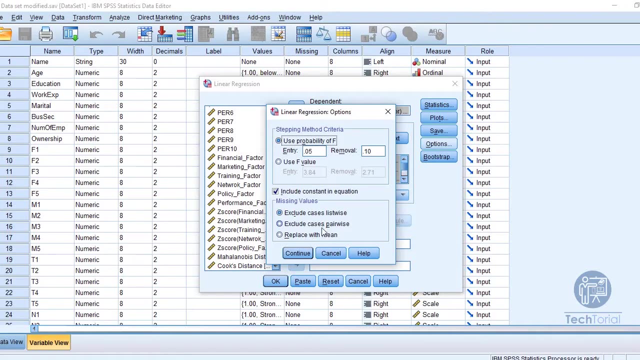 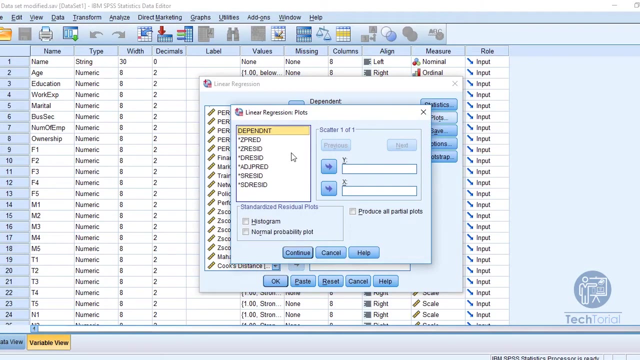 option voice diagnostics and outlets outside three standard deviations. press the continue button in the options button in the missing values to exclude cases. pairwise must be ticked in the plot section. the Z RESID should be in the Y box and ZPRED in the X box. in the standardized residual plots you have to: 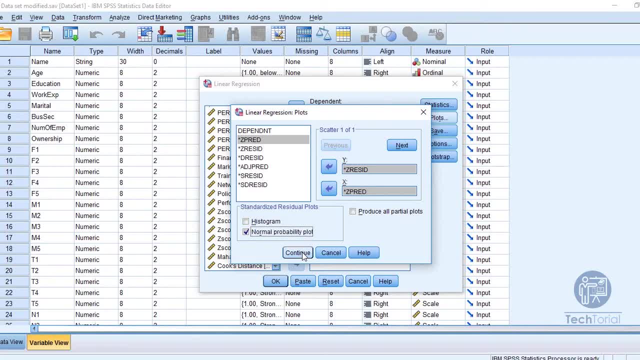 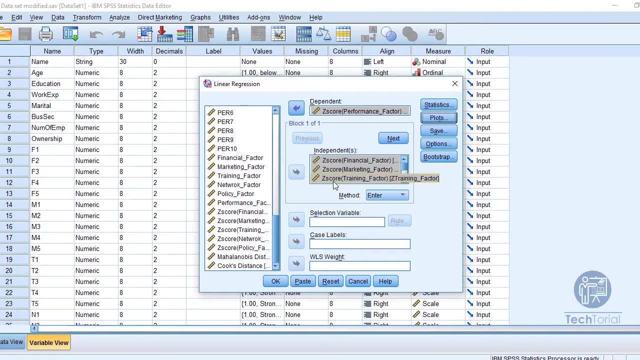 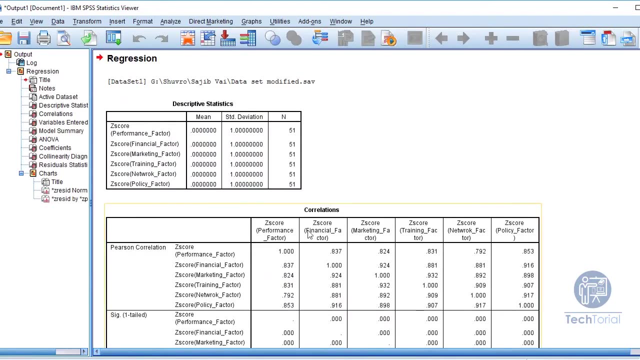 put the normal probability plot. press the continue button. now all are set to do the multiple regression analysis. press ok and you will have the results. now you can see there is a model summary. and you can see there is a model summary. and you can see there is a model summary and. 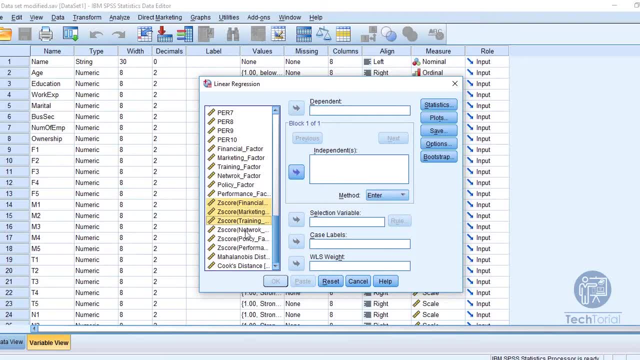 Now I am putting all of the independent variables into the independent variable box And the dependent variable and the dependent variable box. Now you have to make sure that all of the values of those independent and dependent variables must be in the standardized values, because no non-normal data can be used for multiple regression analysis. So 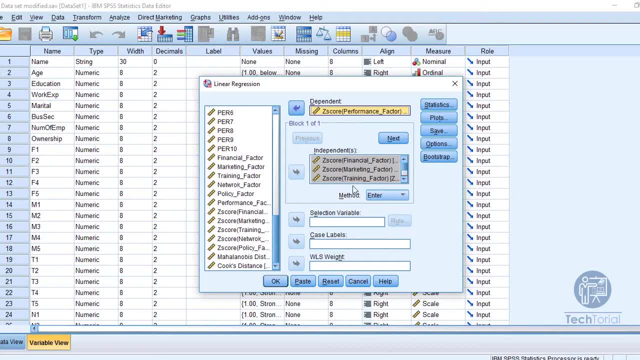 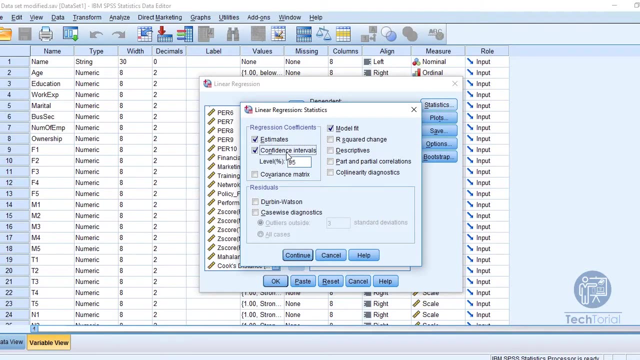 let's get to the method Now. in the method option the enter mode must be selected. Next you have to make sure in the statistics section There are estimates, the confidence intervals, model, fit descriptive part and partial correlations and collinearity diagnostics must be ticked In the residual. 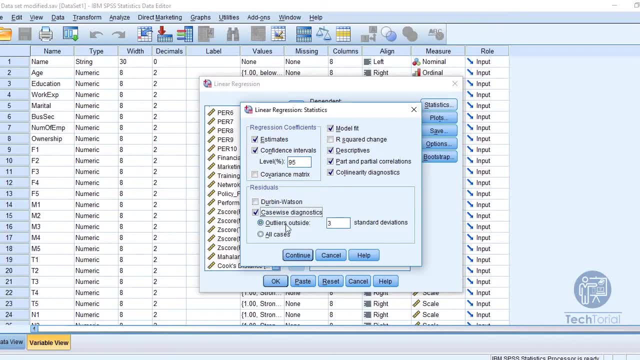 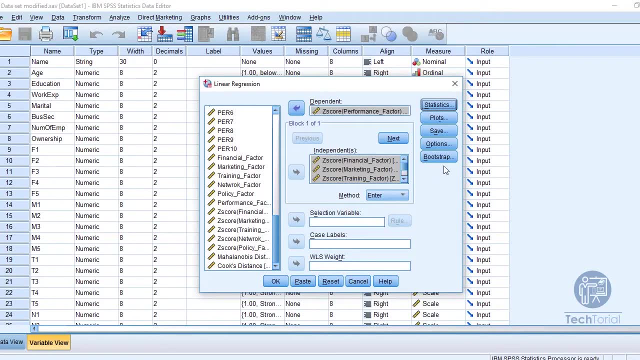 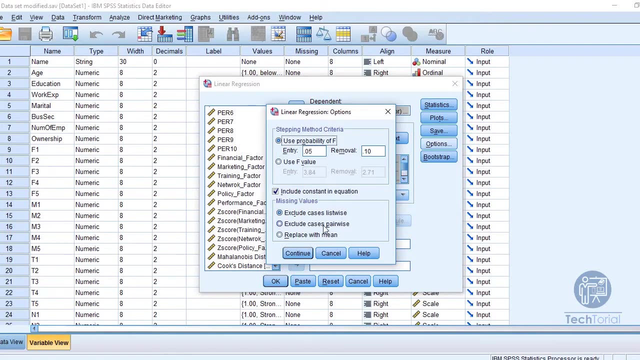 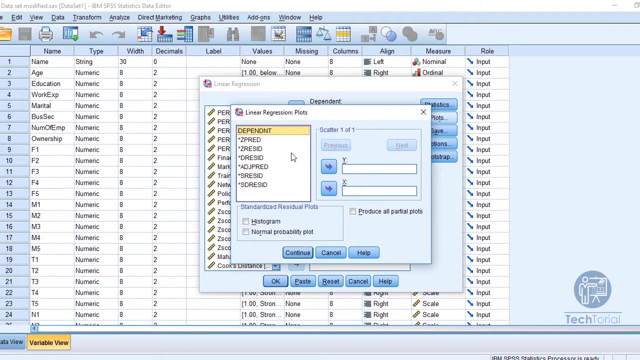 option. tick the casework, voice diagnostics and outlets outside three standard deviations. press the continue button in the options button in the missing values to exclude cases. pairwise must be ticked in the plot section. the Z RESID should be in the Y box and ZPRED in the X box. in the standardized residual plots you have to. 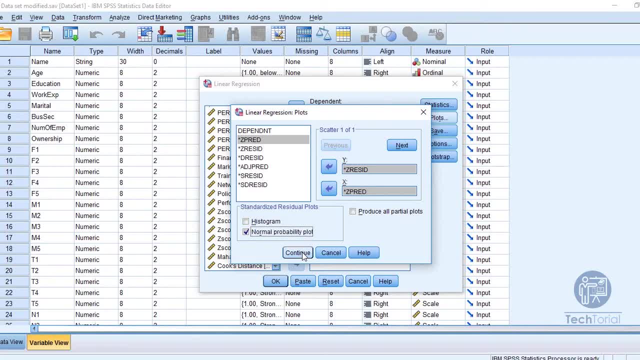 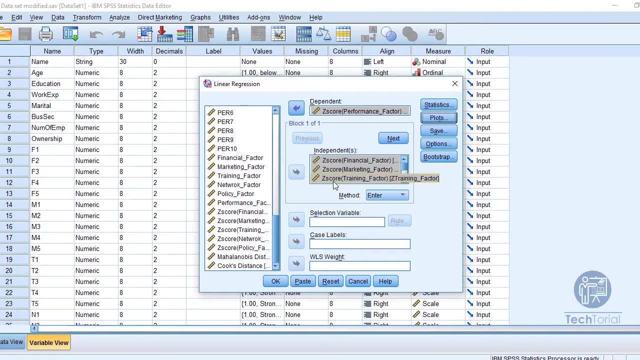 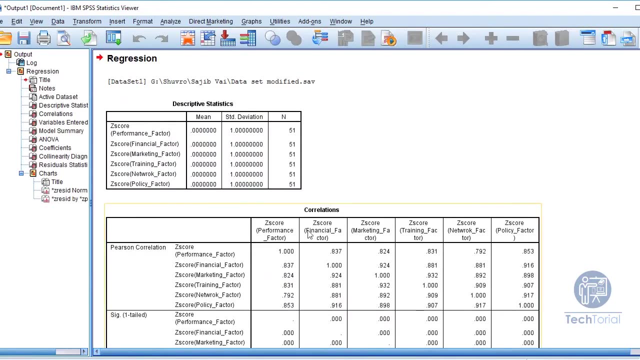 put the normal probability plot. press the continue button. now all are set to do the multiple regression analysis. press ok and you will have the results. now you can see there is a model summary. and you can see there is a model summary. and you can see there is a model summary and. 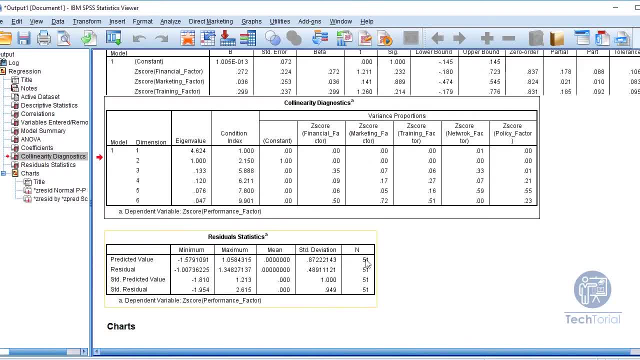 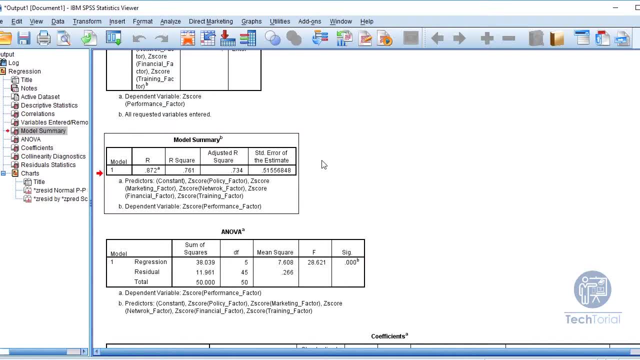 over the coefficients culinary diagnosis takes. all of the results are there. now we have to see what results means what. yes, we are going to interpret those results. in the model summary section there are some results. we have to see what the R square value means here. the R square value is 0.761, that's. 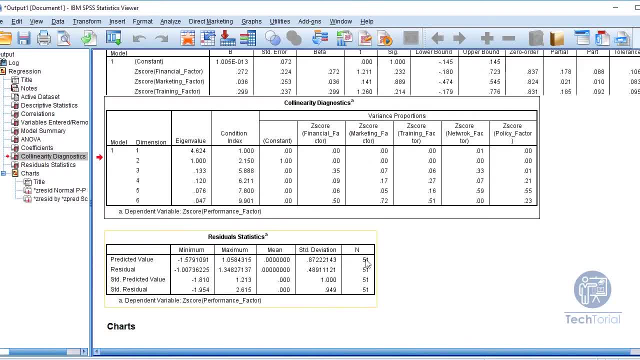 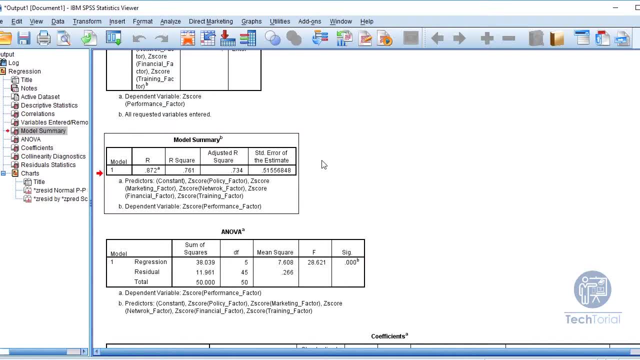 over the coefficients unbelievably sticks. all of the results are there. now we have to see what results means what. yes, we are going to interpret those results. in the model summary section there are some results. we have to see what the R square value means here. the R square value is 0.761. that 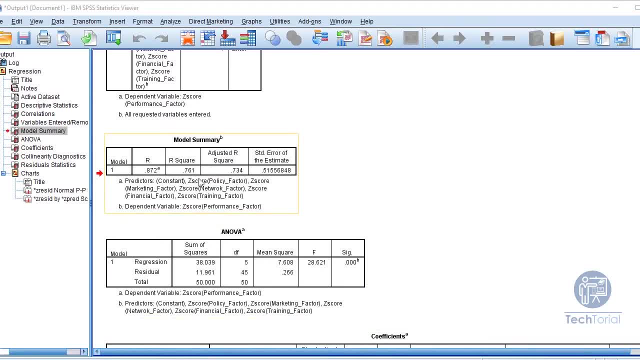 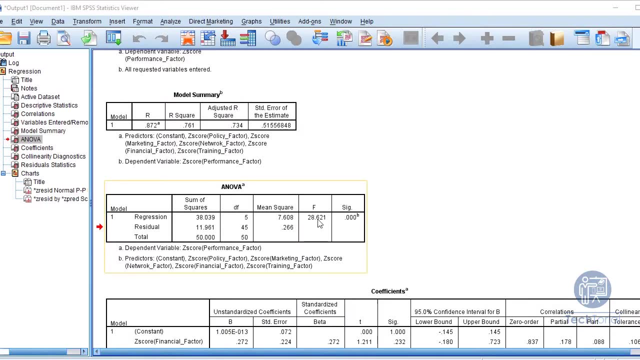 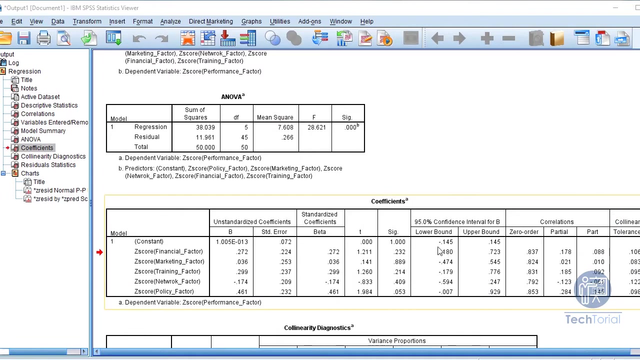 means. that means seventy six point ten percent of the dependent variable can be explained by the model or the dependent variable. in the ANOVA box you can see the significance level is point zero, zero, zero. so you can tell that the model you have used is statistically significant. now there is a table called 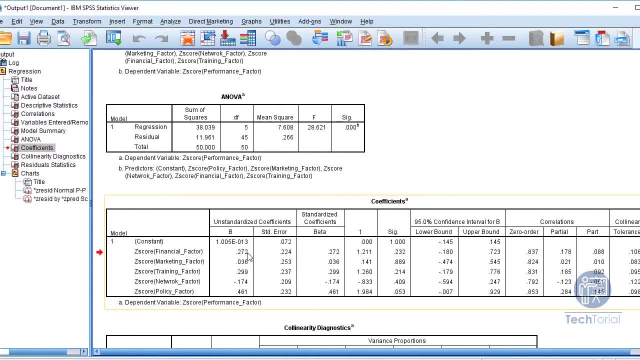 coefficients. this will tell us which independent variables are contributing how much to the model. now in the standardized coefficient box there is a column beta. the more the beta value is, the more significant contribution. the independent value is the more significant contribution the more the variable is contributing. here the highest beta is for this variable. sorry. 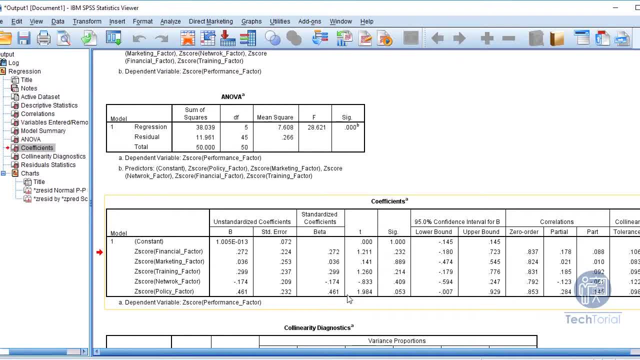 this variable and is point four, six, one. and you have to see another thing that is called significant. now, if the significance level is point zero five or less than point zero five, then it's contributing unique to the model. here we can see there is no variable which is contributing. 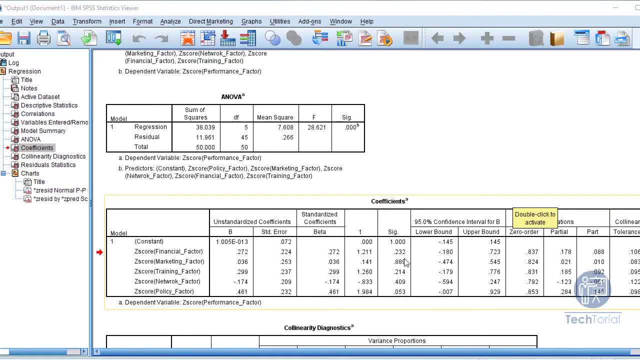 uniquely to the model, significantly unique to the model here. last variable, which has the highest beta coefficient, but it's not less than the point 0, 5, significance 11. so it's not contributing uniquely significant to the model, but it's quite significant to the model. that's how you have to analyze and 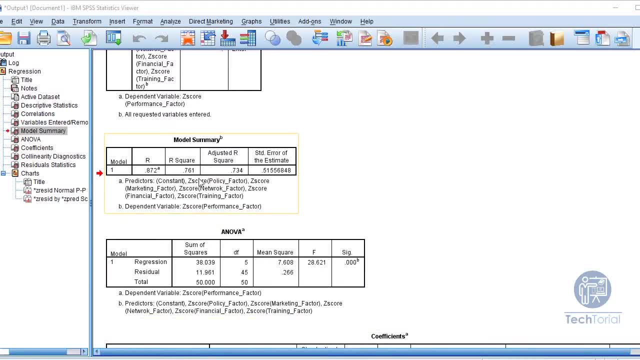 here the R square value is 0.761. that's here the R square value is 0.761. that's means that means 76 point 10% of the means. that means 76 point 10% of the means. that means 76 point 10% of the dependent variable can be explained by: 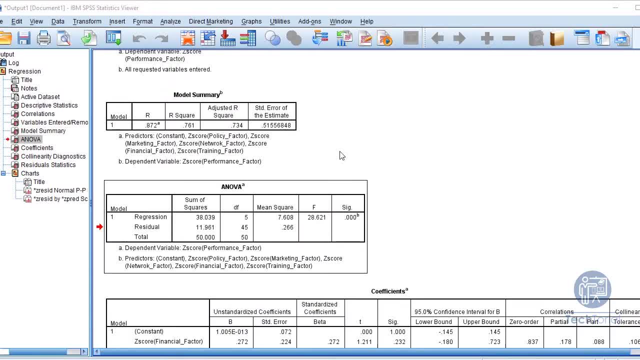 dependent variable can be explained by dependent variable can be explained by the model or the dependent variable in the model or the dependent variable in the model or the dependent variable in the ANOVA box. you can see the the ANOVA box. you can see the. 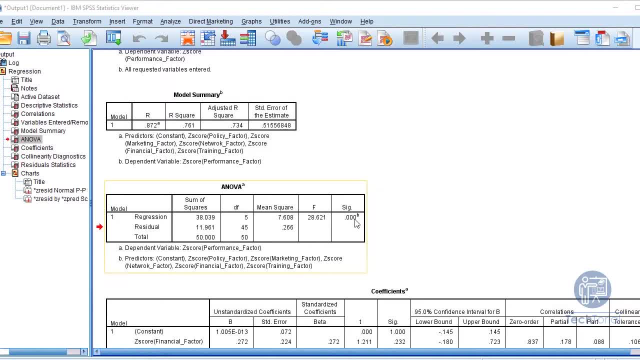 the ANOVA box, you can see the significance level is 0.000. so you can. significance level is 0.000. so you can. significance level is 0.000, so you can tell that the model we have used is. tell that the model we have used is. 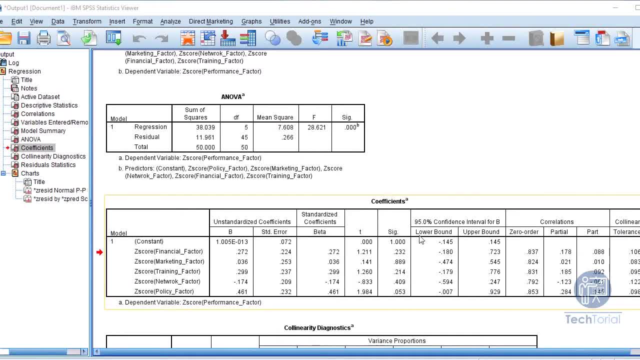 tell that the model we have used is statistically significant. statistically significant: Now there is a table called coefficients. This will tell us which independent variables are contributing how much to the model. Now in the standardized coefficient box there is a column beta. The more the beta value is, the more significant contribution. the 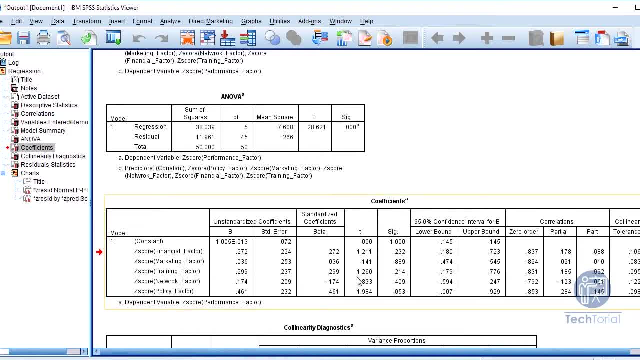 independent variable is contributing Here. the highest beta is for this variable and is 0.461.. And you have to see another thing that is called significant. Now, if the significance level is 0.05 or less than 0.05, then it is contributing. 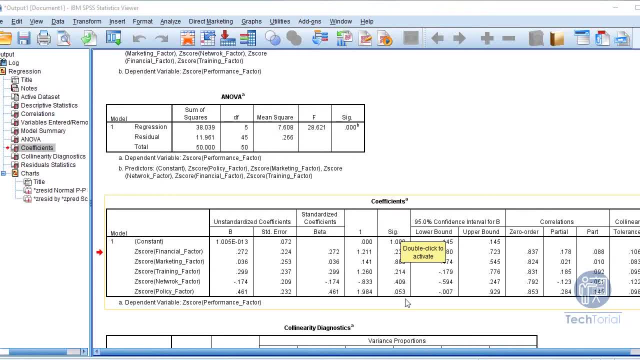 uniquely to the model. Here we can see there is no variable which is contributing uniquely to the model, significantly unique to the model. Here. the last variable, which has the highest beta coefficient, but it's not less than the 0.05 significance level. So it's 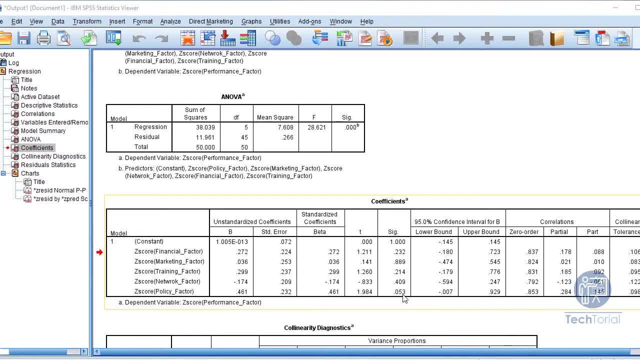 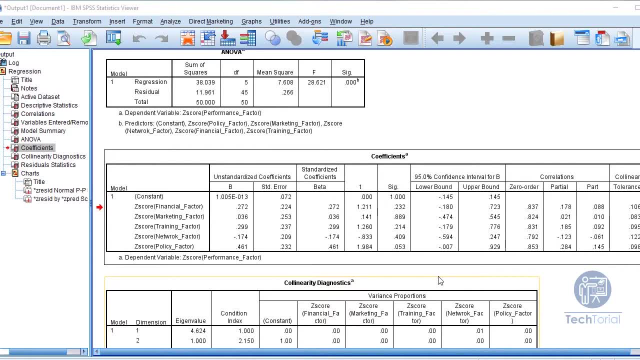 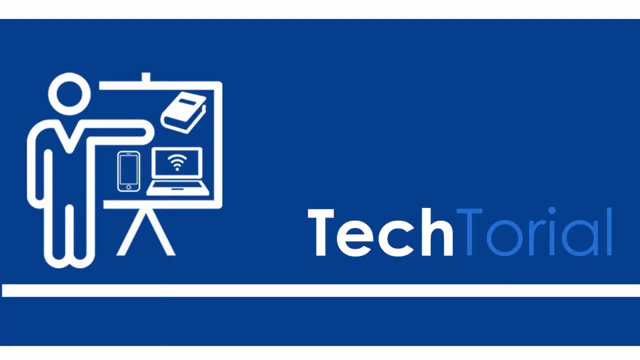 not contributing uniquely significant to the model, But it's quite significant to the model. That's how you have to analyze and interpret the multiple regression analysis. Thanks for watching this video. I am Shubhruv from TechTorial, So if you have any queries,